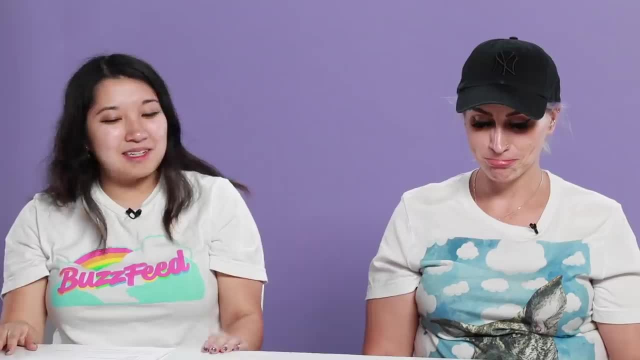 and then I feed her again. She kind of takes care of herself. There are times when I like, I like, try to be like Mummy, let's play, let's hang out, And she's just like, don't talk to me. 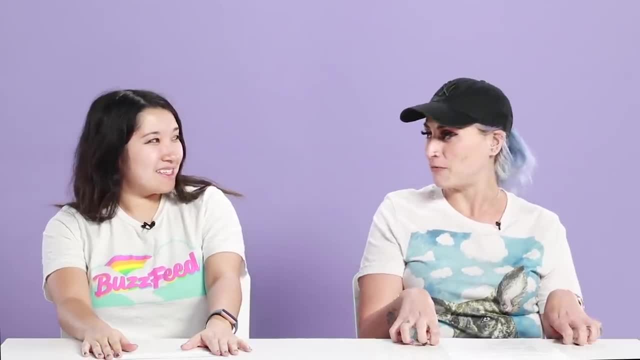 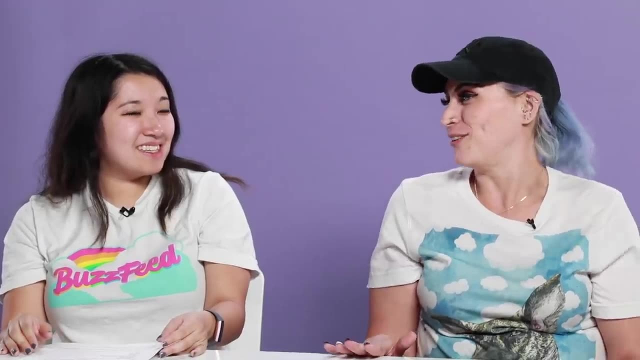 Don't bother me. So the whole video is going to be me begging Mummy to love me. It's possible. It's possible. I think I'm going to be the saddest living creature participating in this video. I don't know why I agreed to do this. 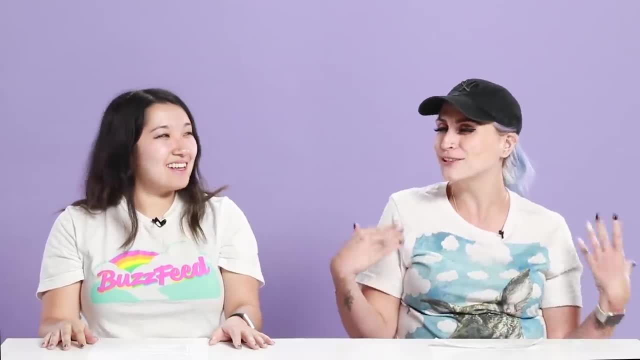 I think at first I thought it was a joke. Like as a joke I was like, yeah, someone take my dog. She's a lot of work. And now I'm like, but that's all I have. I miss having a dog. 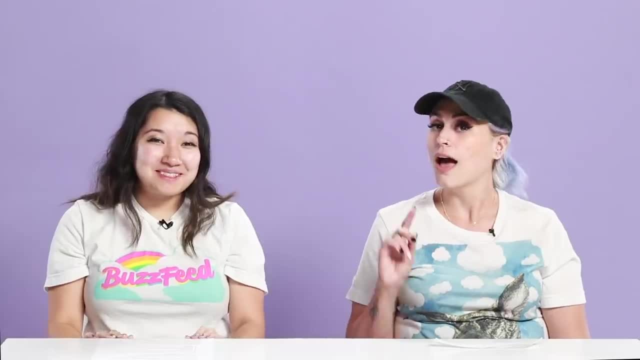 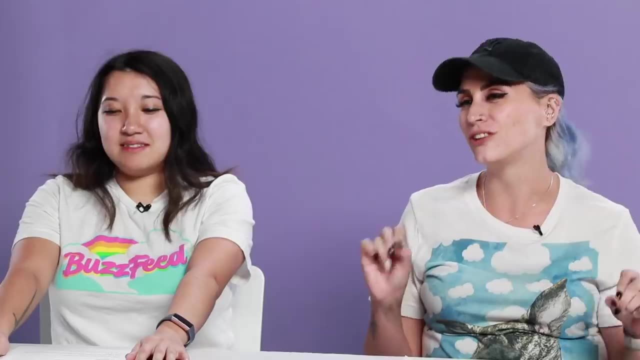 I love having a cat and I love Mummy. I am a dog person as well as a cat person. I also kind of miss the freedom that comes with cats. Like I'm going to run so many errands tomorrow, Oh yeah, Well two. 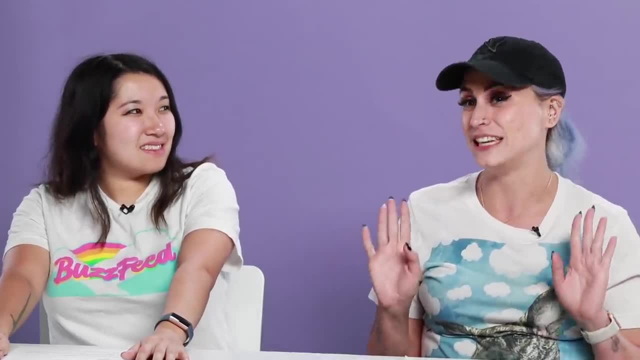 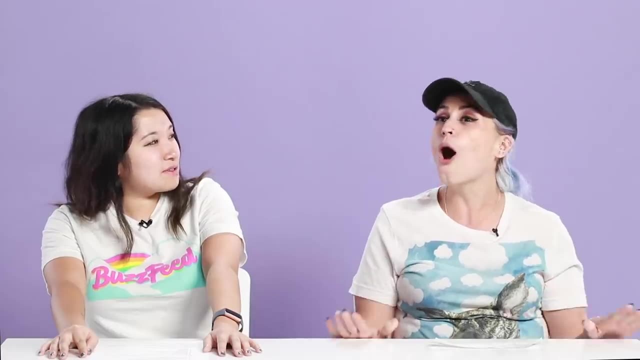 But still, I'm going to leave the house without my dog on a Saturday for the first time in a year. I'm also going to pee with the bathroom door shut for the first time in like a year and change. Does she not like the bathroom door? 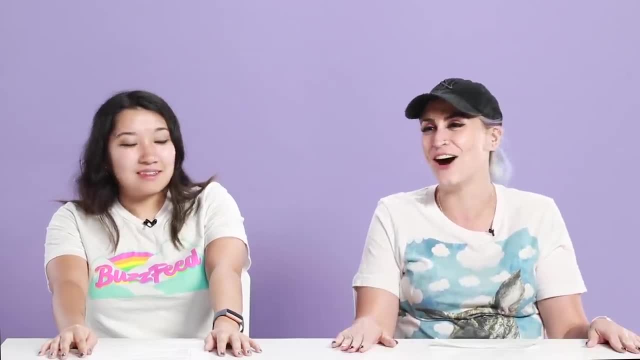 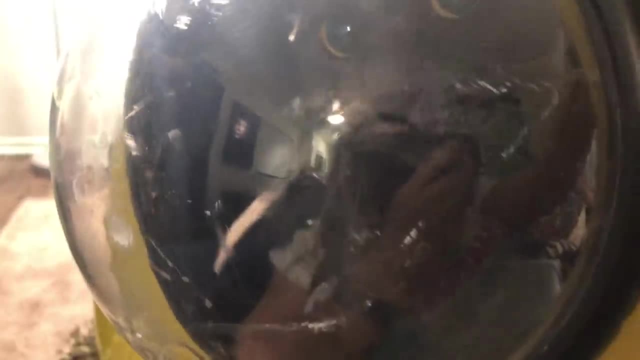 Oh yeah, No, no, don't, Yeah, no, That's it. Yeah, you're not going to pee alone. Sorry, Should have led with that. I love you. It'll be fine, It'll be okay. 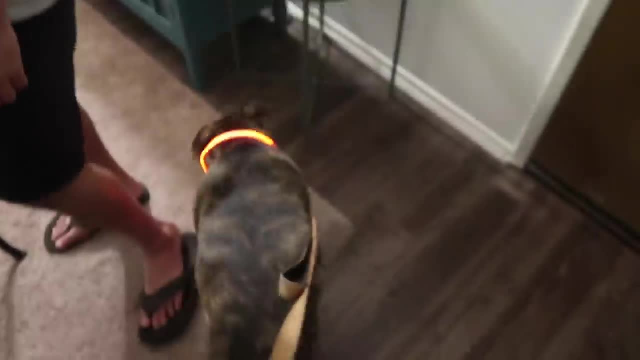 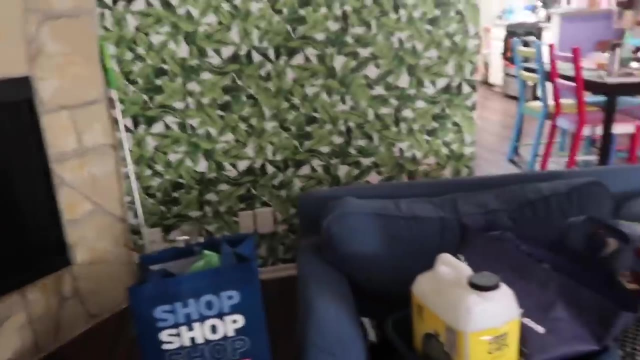 You'll like, Becky, You're not going to the vet, You're going to be okay. Yeah, Are you ready? I'm going to take off your leash, Okay, Oh see, this is off to a great start. Are you afraid of the pinata? 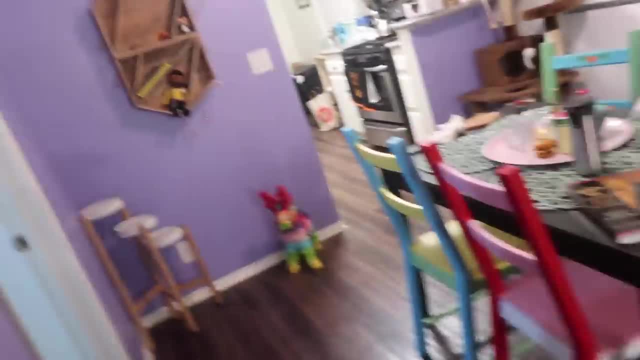 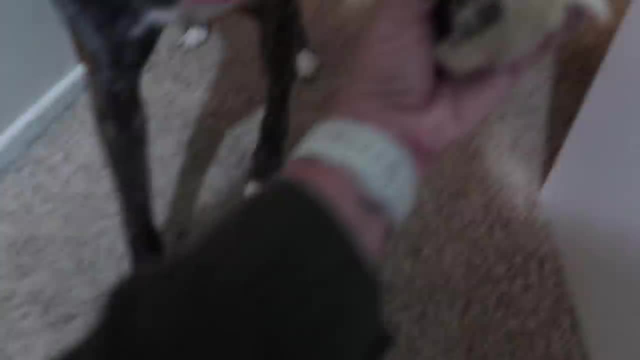 Is she afraid of the pinata Bubba? what is this? What is that? What is it? Oh, you will eat cat toys. Good, Oh, wow, You found another one. Okay, Come on, I love you. 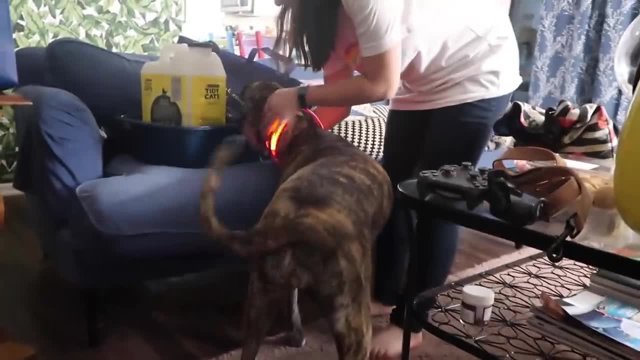 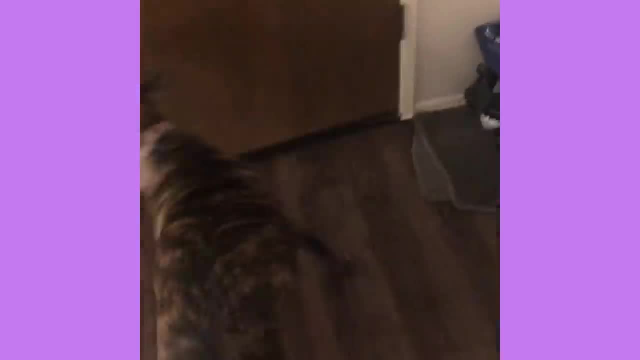 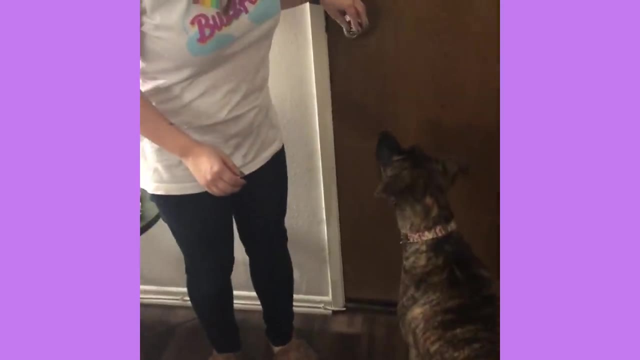 You are my baby, You be good, okay, Okay, Hi, Then I'm leaving you. Hi, Hi, Hi, Hi Hi. Oh, Becky's not here, It's okay, I'm here, I'm your friend. 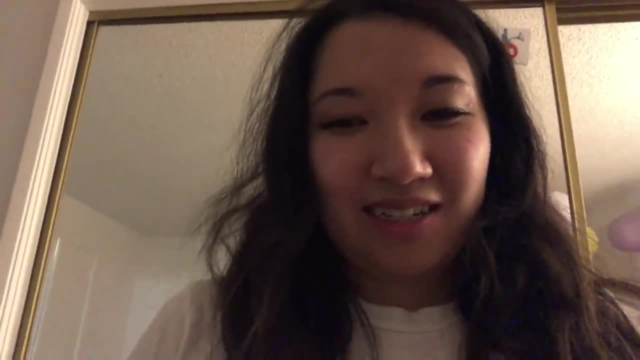 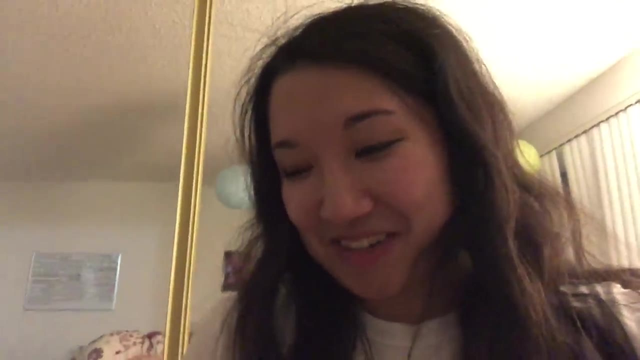 Okay, so Becky's gone and Mabel's here. I'm excited, I'm excited, I am just nervous. But She's not going to like it because I'm not Becky. Okay, I have just dropped off Mabel Monster. 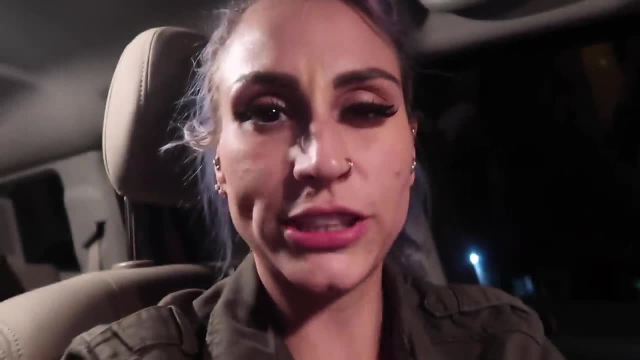 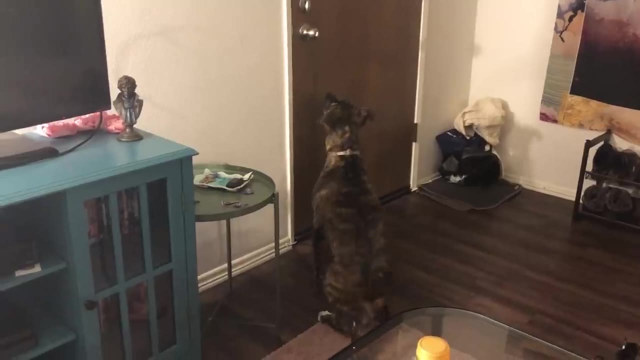 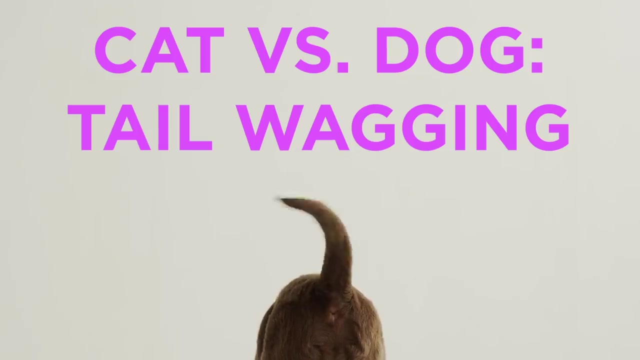 Mommy and I are in the car. I think she's a little afraid she might be going to the vet, So I'm hoping my apartment is a nice surprise. Oh, she misses Becky. Poor kid. I don't know what it means when cats wag their tails. 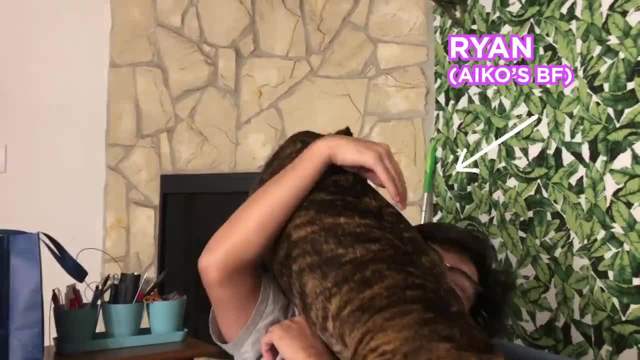 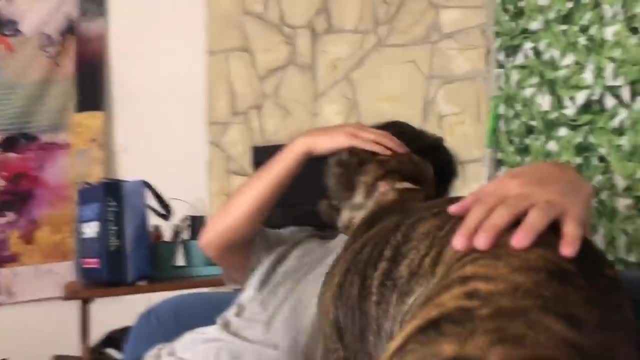 Do cats wag their tails when they're happy? Is that a thing, Mabel? Oh my god, are you okay, Mabel, I'm okay, This is okay. This is a lot, but, to be honest, kind of nice. 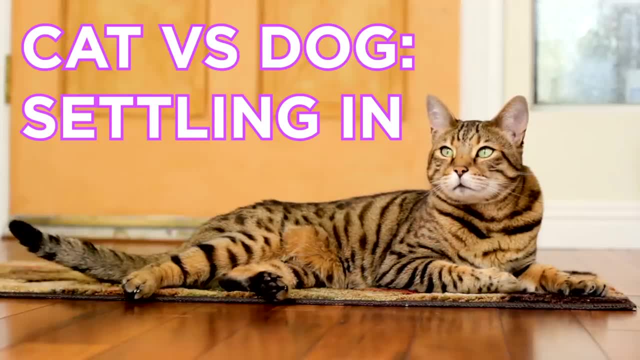 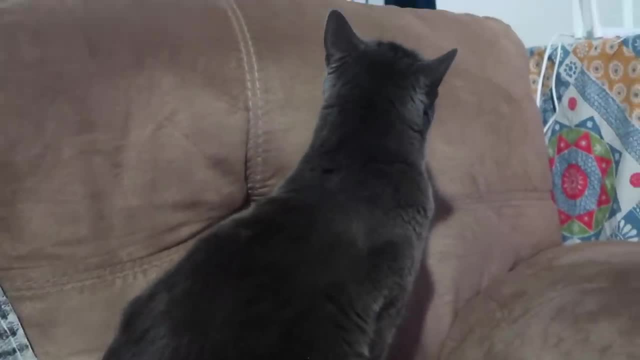 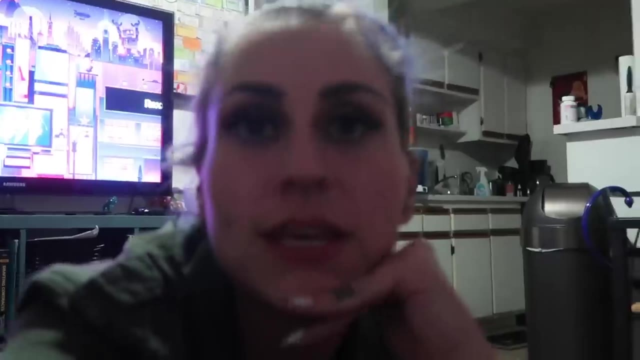 I don't get a lot of snuggles. Okay, I'm going to let you look around while I set up your stuff. Deal, Okay, Okay. So here's the other thing I think I probably, maybe sort of neglected to mention. 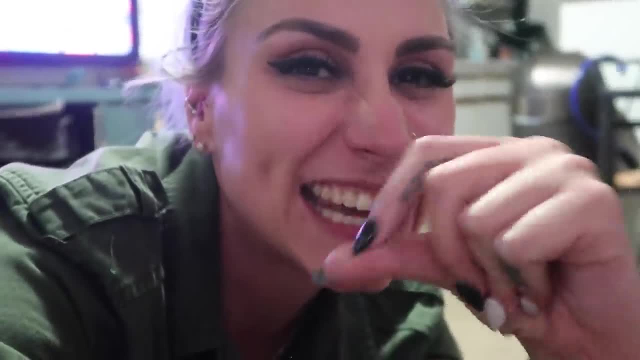 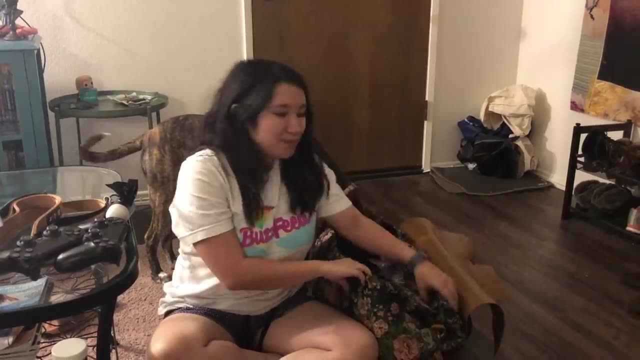 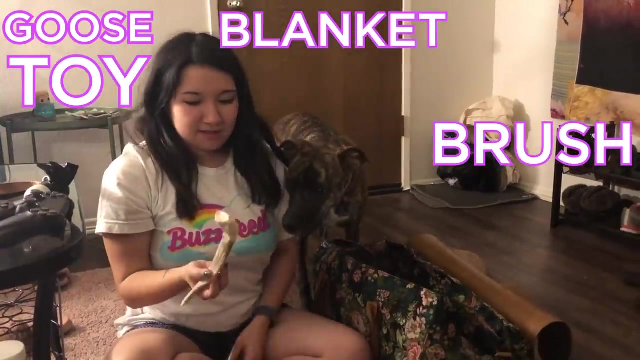 I am just the teeny, tiny, slightest bit allergic to cats. I'm going to take some Benadryl and we're going to have some fun, yeah. So Becky gave me this giant bag. So this is a goose toy, your blanket, I think a brush. 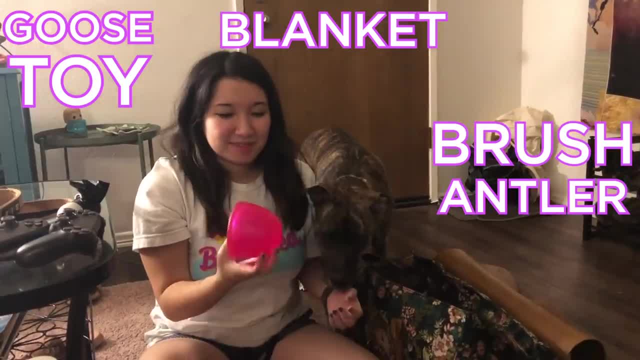 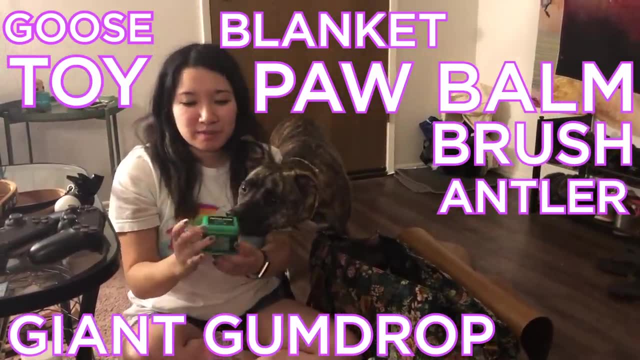 What is this, Antler, Antler, Oh, okay, This looks like a giant gumdrop. Oh, that's the bomb that she was talking about. Apparently, Mabel gets paw bomb. It looks like your toothbrush and toothpaste. 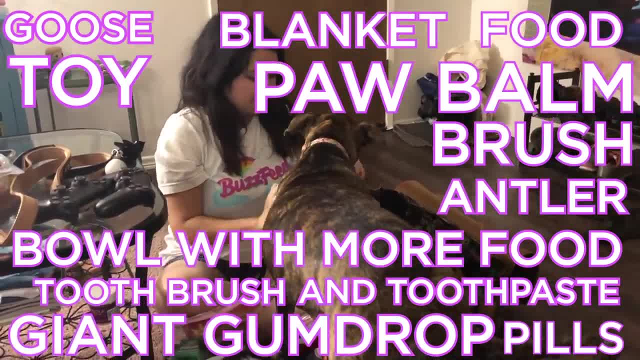 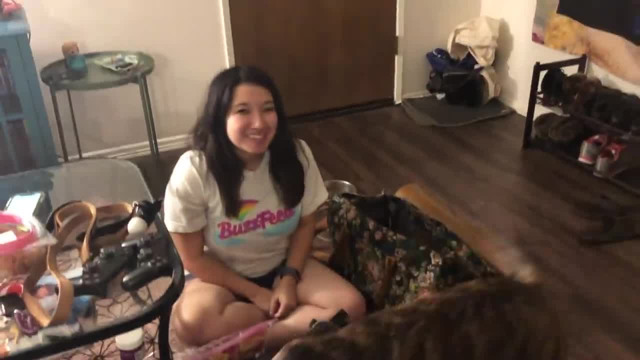 Your pill. We got food bowl that has food in it. I bet that's your water bowl. This looks like her harness. That's a lot of stuff. I'm not going to lie For one night. that's a lot of stuff. 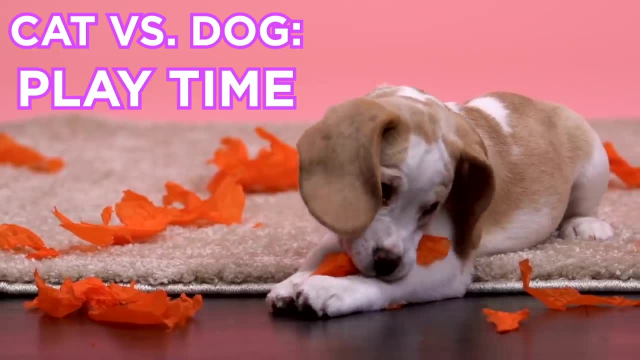 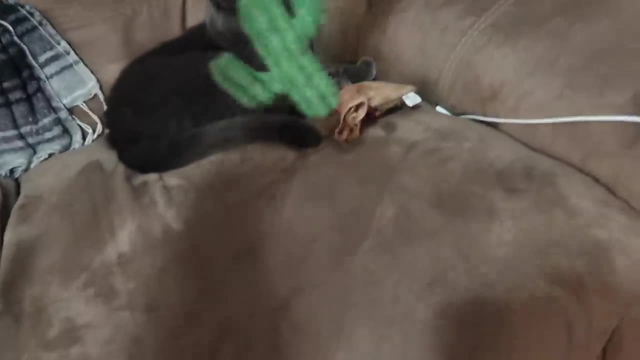 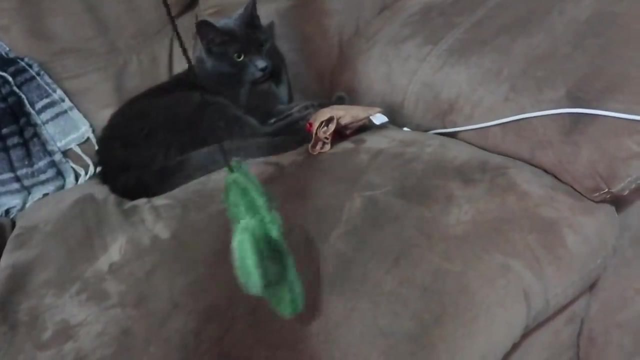 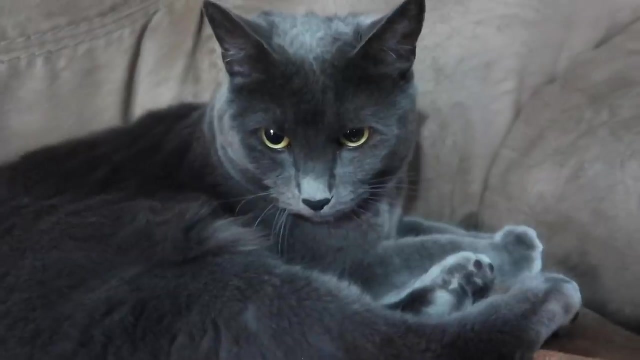 I feel prepared. Mommy has no interest in playing with me right now, So this is going well. She is letting me pet her Lots of good pets. You can definitely tell she's a little nervous. She's not sure what to make of this place, which is fair. 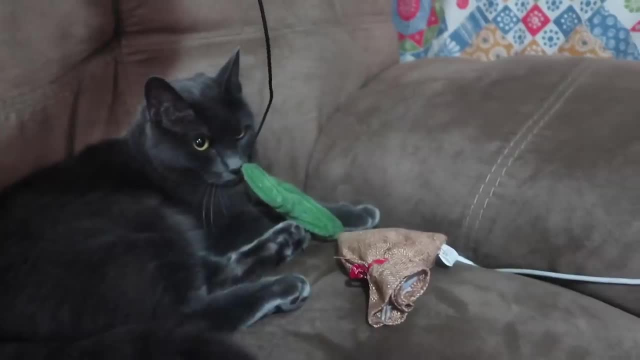 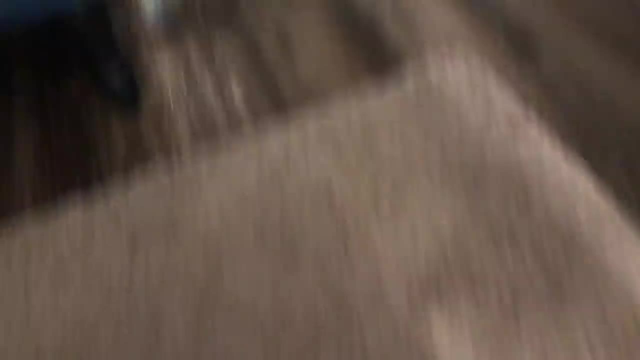 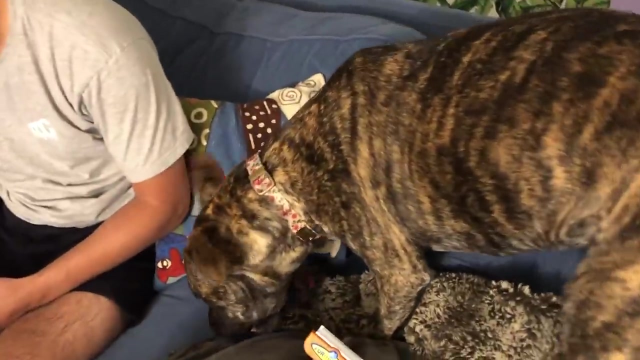 It's new and it smells like dog. She's not amused by my bull. Hey, Mabel, that's mommy's toy. Okay, Mabel stole one of mommy's toys. Can I have that bag please? Oh, mommy liked that. 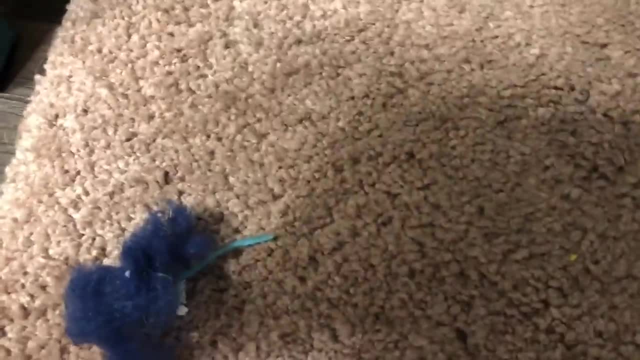 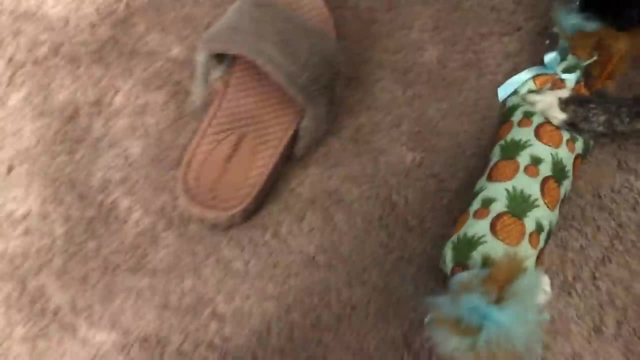 Mabel, I told you that's mommy's. Hey, give me that. That's a feather. You don't want that. Okay, Mabel is just taking all of mommy's toys. Oh, stop, Stop it, That's a feather. 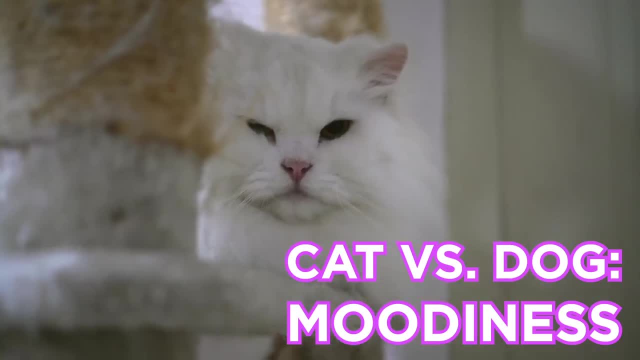 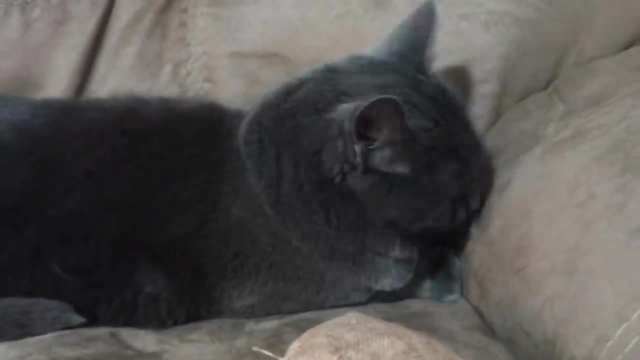 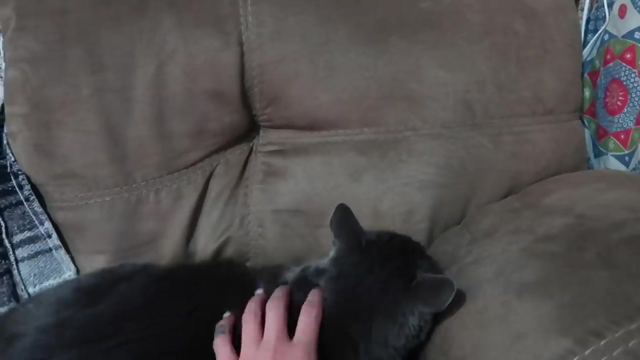 I'm going to be going to PetSmart after this. I have just been informed that a light tail wag means you're probably annoyed with me. Based on your body language, that is probably pretty accurate. So what I'm going to do? I'm going to go take a shower and I'm going to give you the whole. 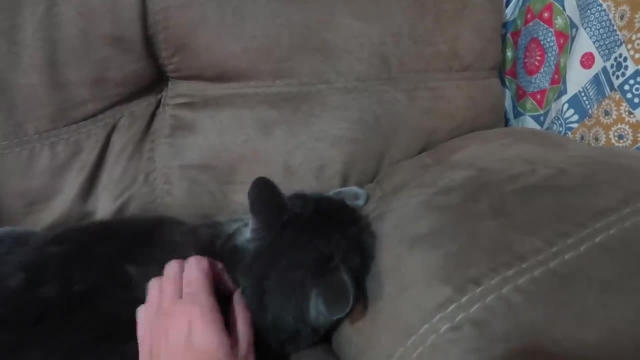 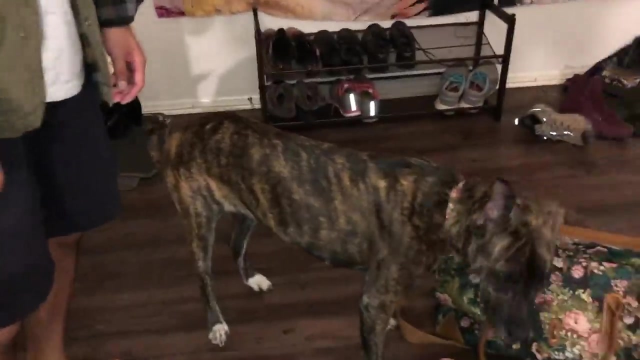 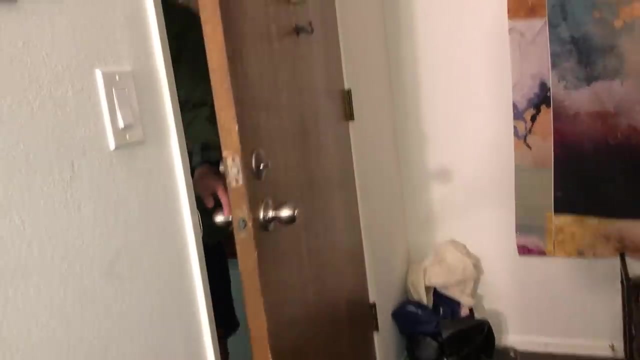 space to yourself to get comfy and to relax and to explore and figure out what you need. Sound good, Okay, Stay fine, Mabel, It's just me, It's just us now. I mean It's just us now. Aww, it's okay. 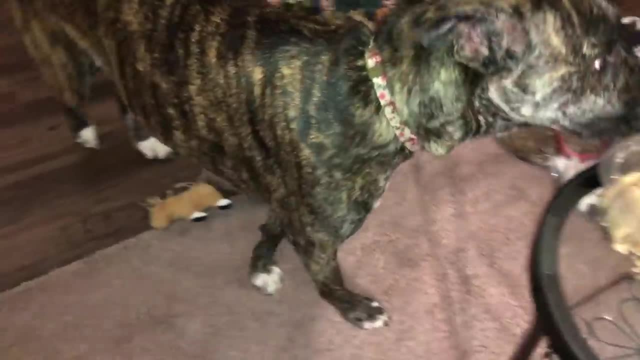 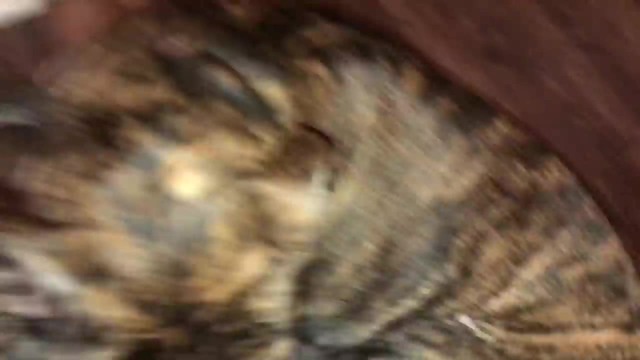 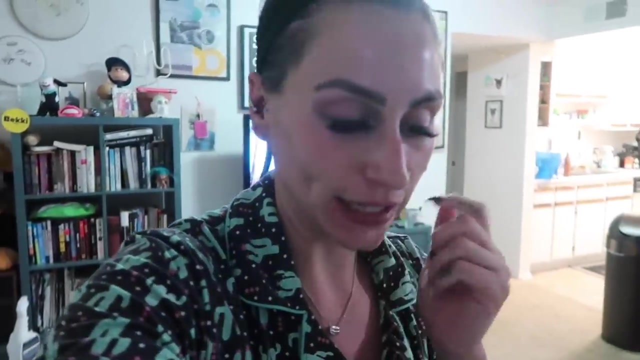 I was just joking. Oh no, oh no, Okay, it's fine. It's fine. Mabel really liked Ryan, and now Ryan is gone. It's okay. Cats Mommy has found her place to hide for the evening. 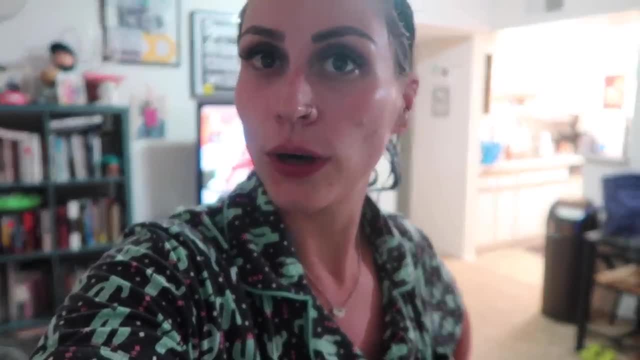 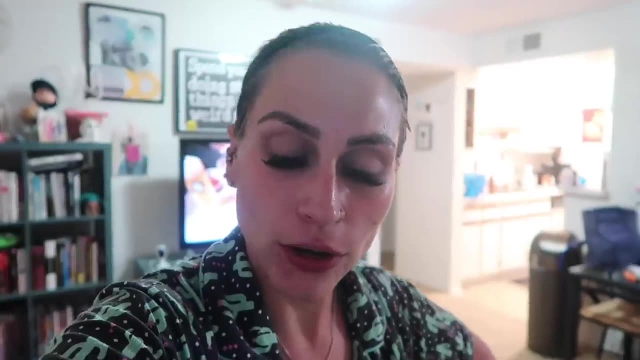 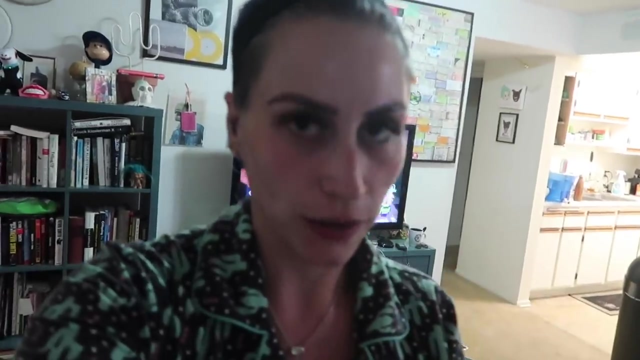 I don't know how she got there. I don't know how we're going to get her out. If we're ever gonna get her out, Yep, nothing, I moved the couch out just a little. I'm not gonna force her out. 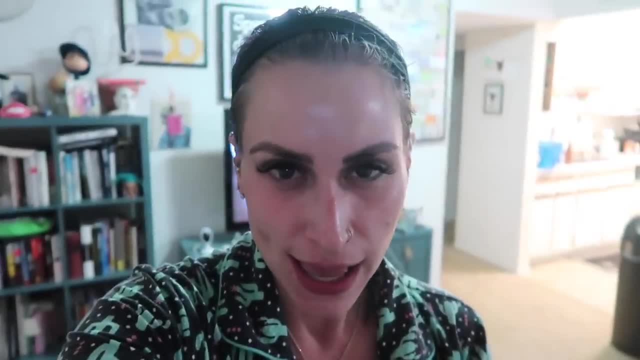 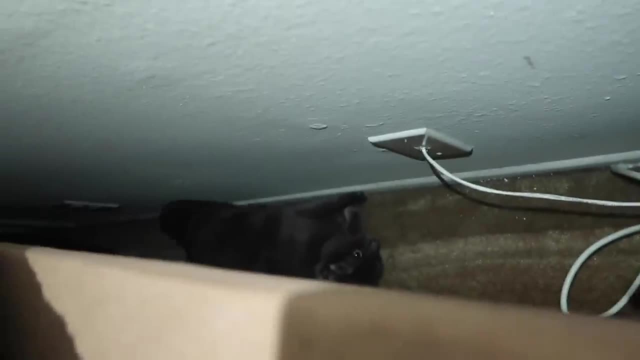 but I want her to be able to get out if she so chooses, And I don't even know how she fit back there. But mommy is alive and well and just chilling hiding behind the couch, So that is where we're gonna let her be for a little bit. 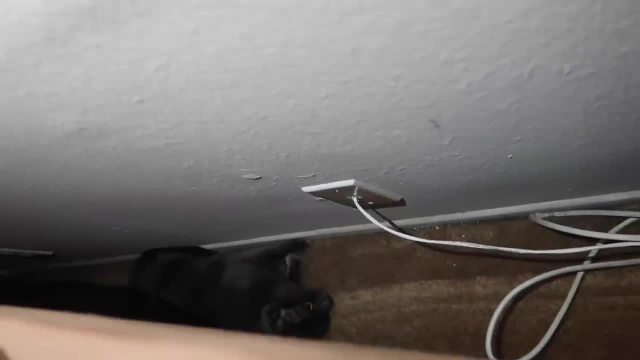 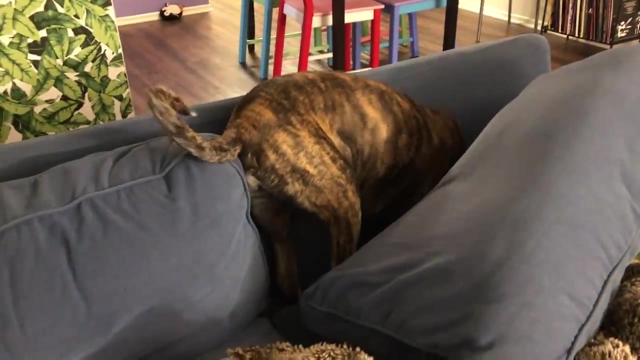 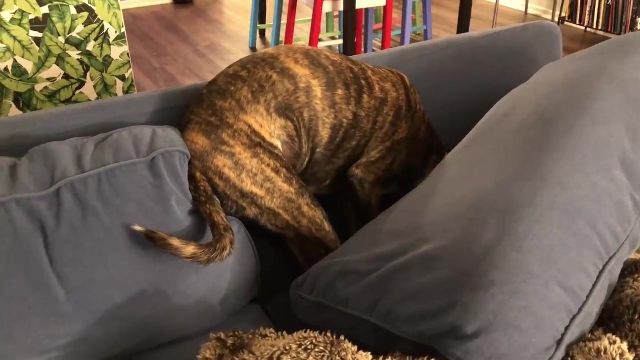 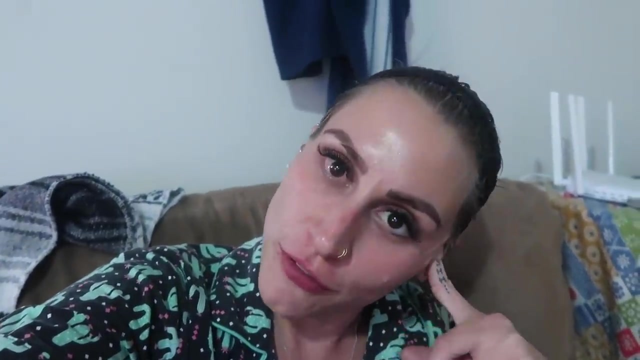 And I'm gonna. I don't know what I'm gonna do. I'm gonna be alone on a Friday night at 9 pm. Um, excuse me, that's my couch. Hello, I was recently talking to one of my friends who is a cat owner. 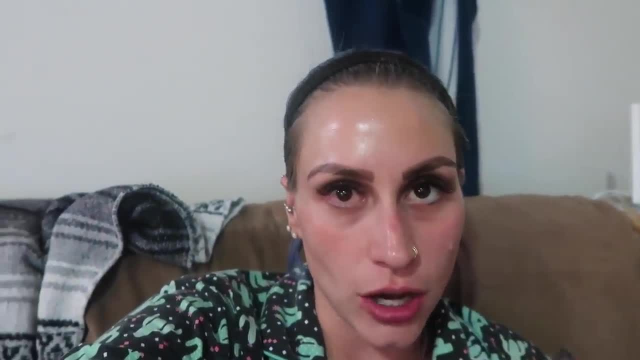 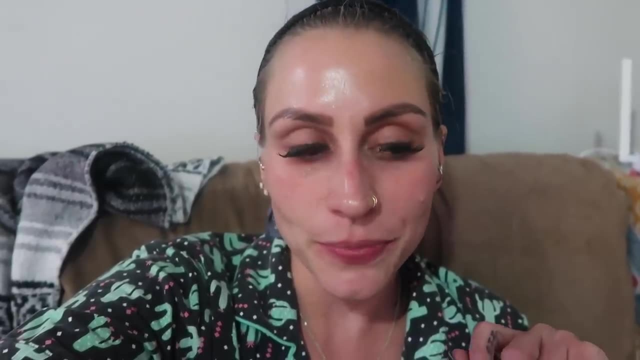 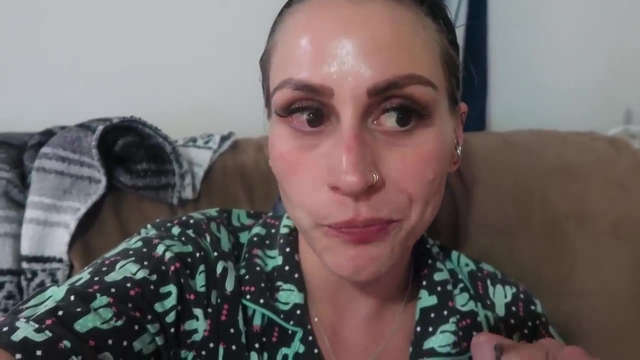 She told me that dogs tend to attach to people and cats tend to attach to places. Taking mommy out of her home base might be setting her off a little bit, which is okay. New places are scary. She's only been here a couple hours. 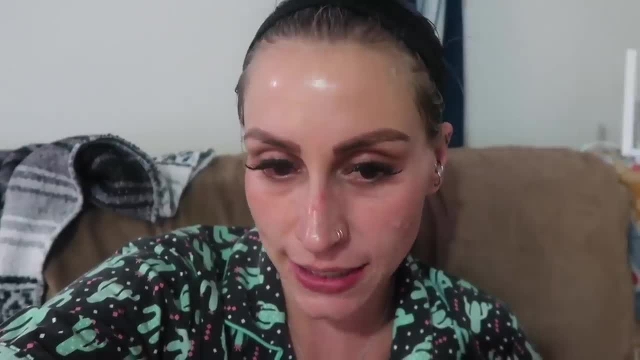 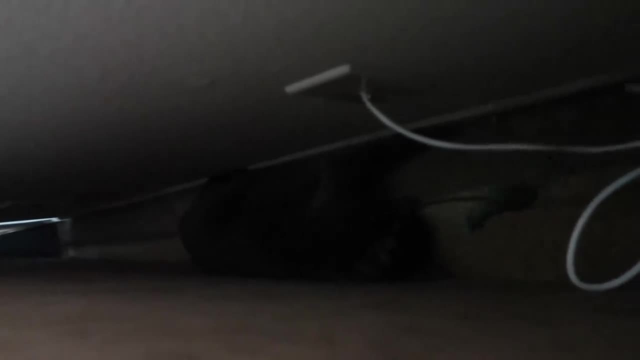 I will say this is not all cats. I have had cats come over and stay here. I don't know if cats do treats. I don't like this honey realm, Not one bit. This would be good for our family, I promise. 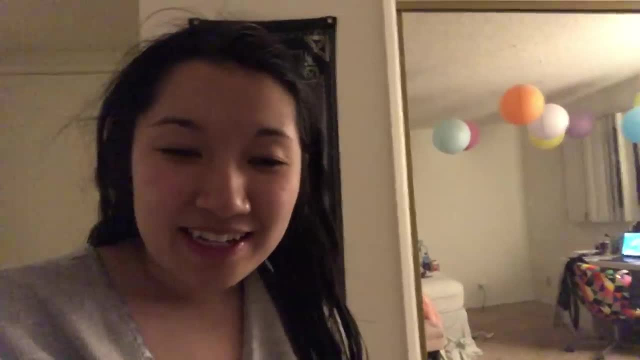 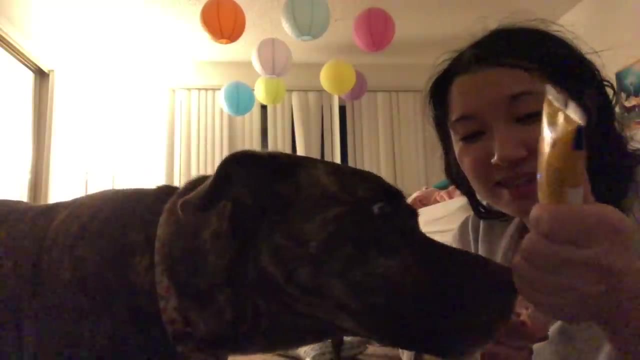 I have just showered and now I'm going to do the night routine that Becky has for Mabel. This is Becky's toothbrush and toothpaste for Mabel. Mabel has like beautiful teeth. Excuse me, Excuse me. 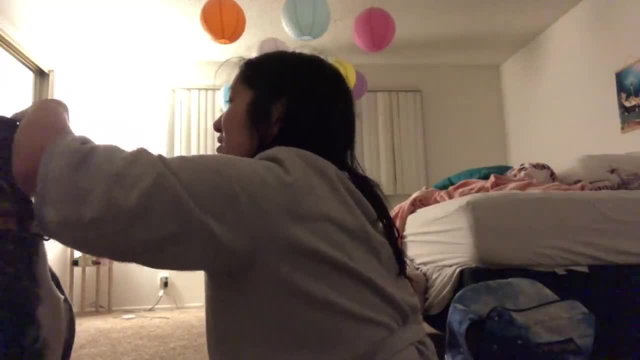 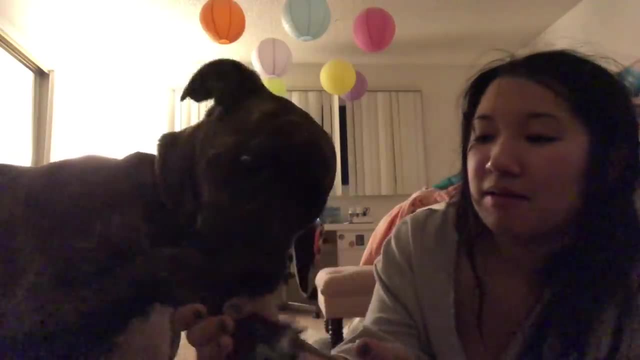 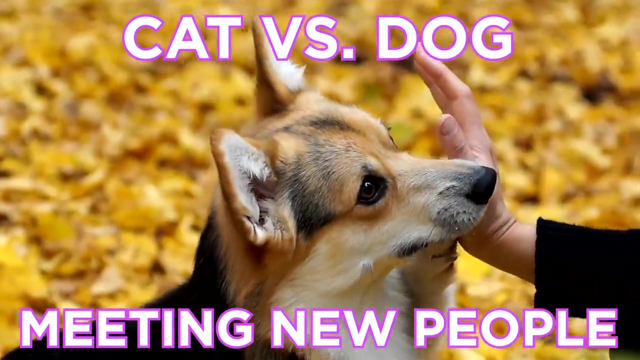 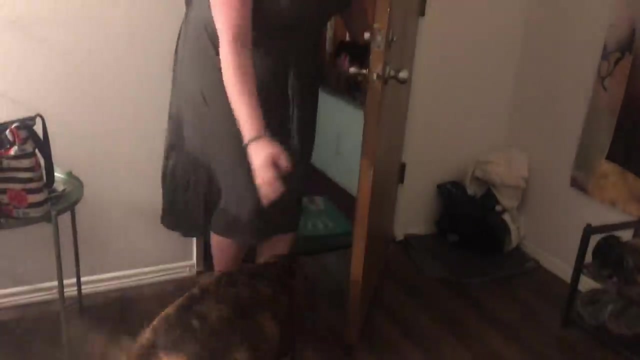 Excuse me correct? Does this hurt? Please tell me if I'm hurting. Oh, okay, You're fine, right? Am I doing it right? I'm doing it right, right, Oh, I'm sorry, Oh my gosh. Oh, hi, honey. Oh, I don't want you to leave. No, no, no, Oh my gosh. Jesus Christ. 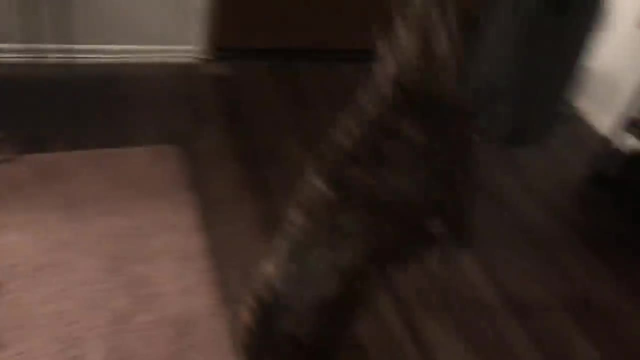 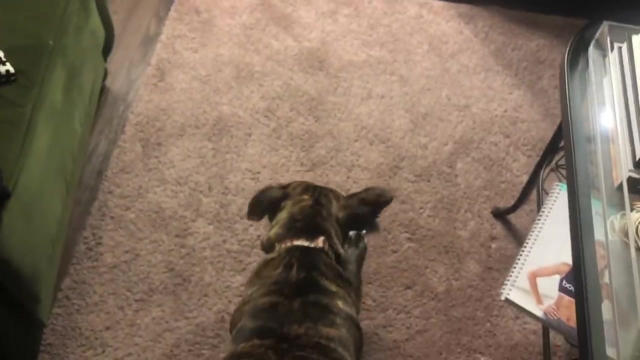 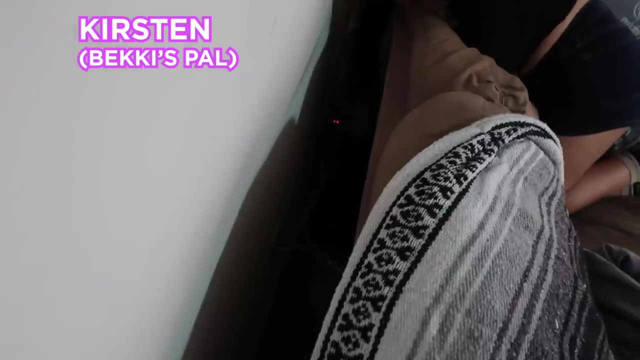 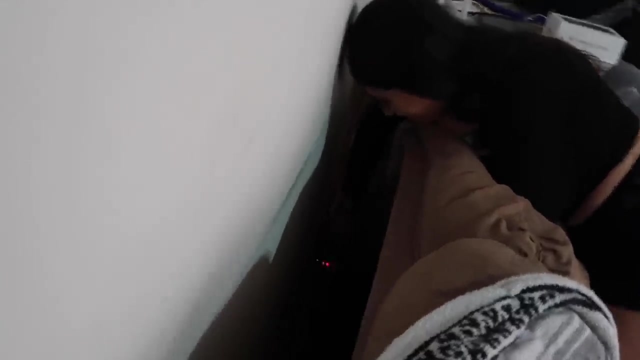 Okay, babe, Let's go. No, that's like flying leaps. Holy shit He's doing. okay, That's actually mommy's toy. How do you pet a cat that won't come out from hiding? Mommy obviously wants to be pet. 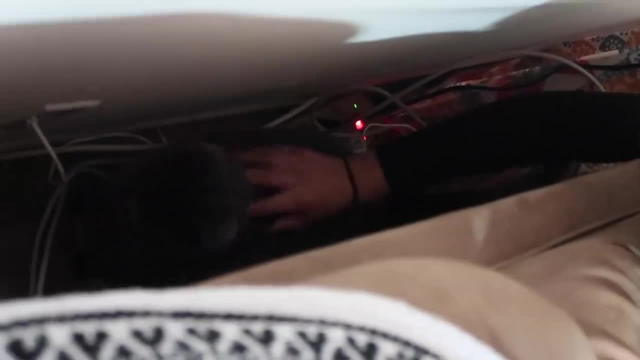 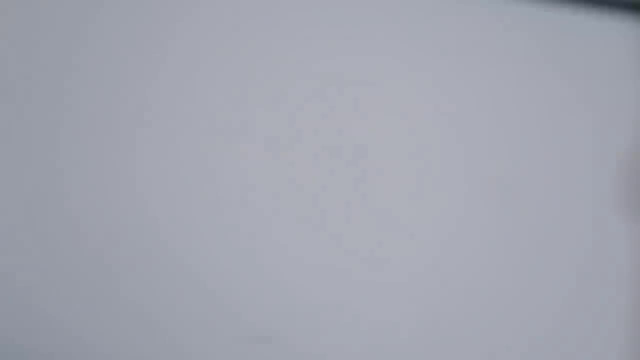 Mommy, Mommy just likes to make you work for it. He's going to let them do their own thing, but you have to let them come to you. Okay, Mommy, Mommy, I just want you to love me. 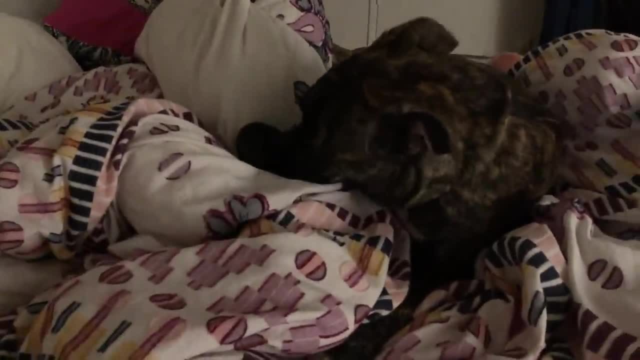 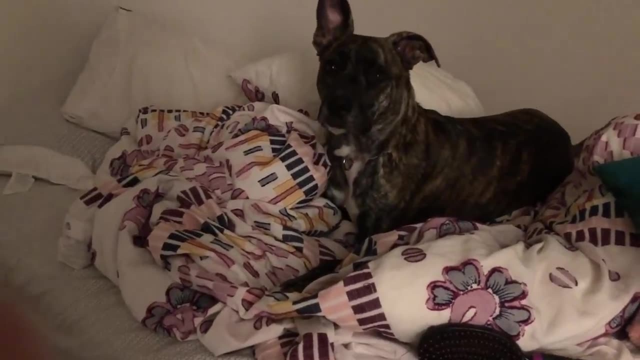 So, Mabel, are you joining me in bed? Mommy usually sleeps on this ottoman right here. I think she's sleeping here tonight. No, I've been told you're snuggly, All right. Good night, Mabel. 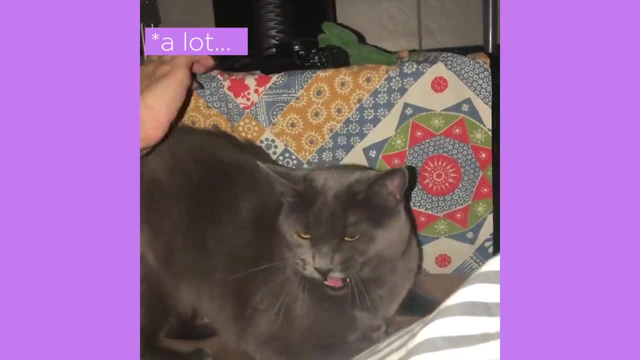 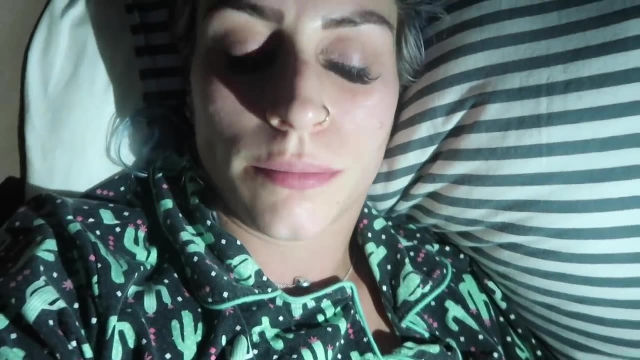 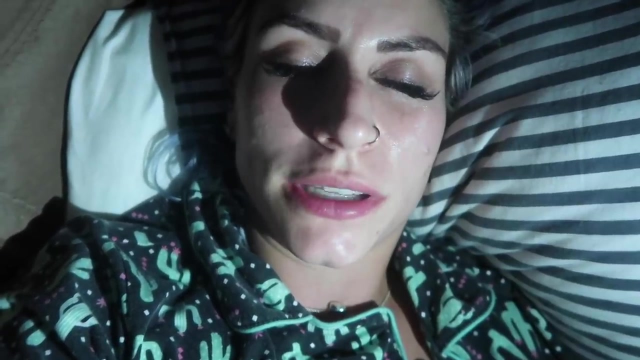 I keep getting woken up to meows, Those meows. It's like 1 am And mommy has decided she has a lot to say. I'm not sure what she wants from me, I don't know, But I think it's a good sign. 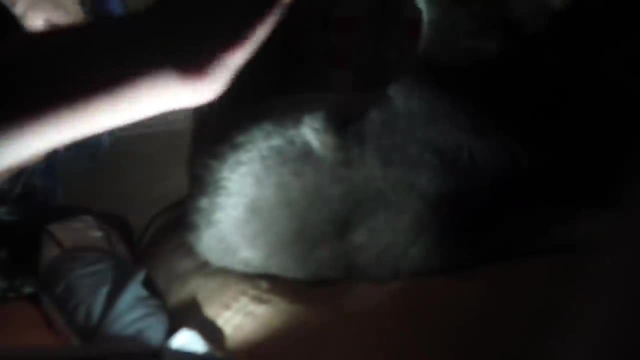 I don't know, I'm tired. It is now 2 o'clock in the morning. I've been woken up again to pet the cat. Just wasn't expecting to be woken up every hour for a pet, but it's like having Mabel. 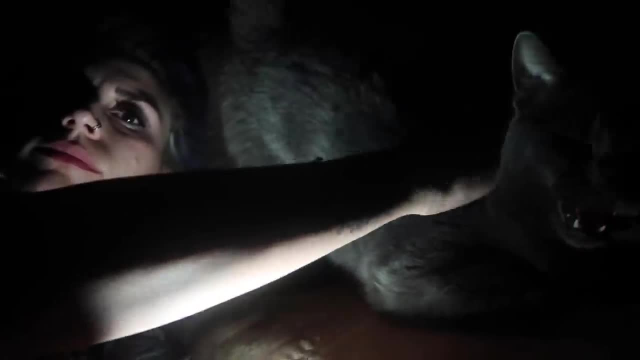 here Just a little louder. It's 6.30.. I usually wake up at 3.30.. I'm not sure if you can hear me or if it's just me. I'm just not sure. I'm not sure if it's Mabel. 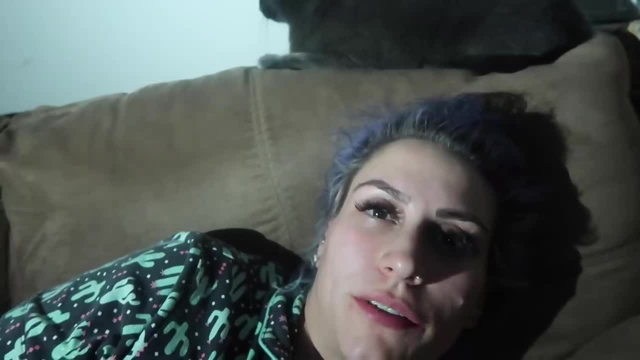 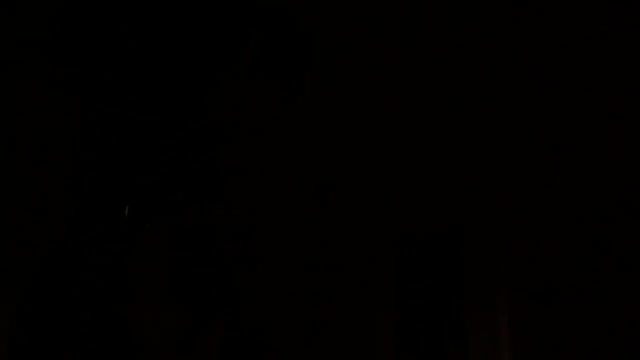 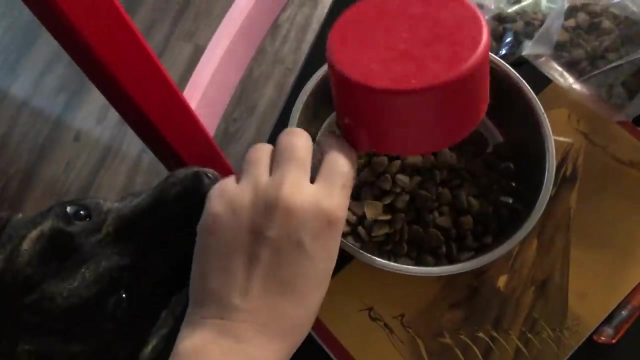 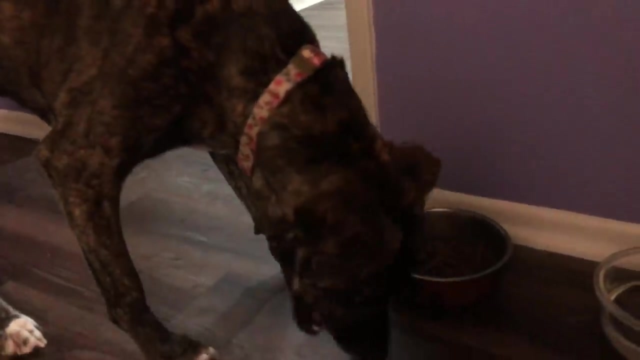 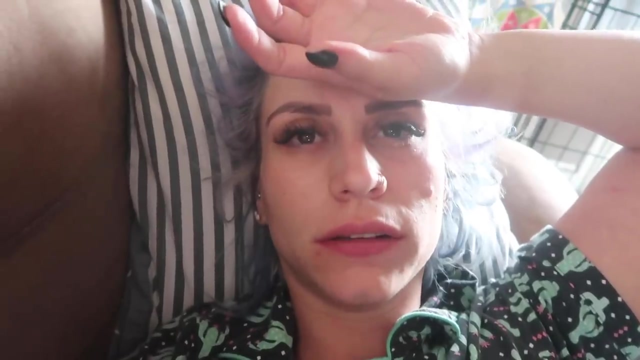 I don't really know if it's that bad, But someone is excited. It's good to see you too. Time to feed her, That's a good girl. Mommy spent all night meowing, Just constantly meowing. I'll probably Google to see what that actually means. 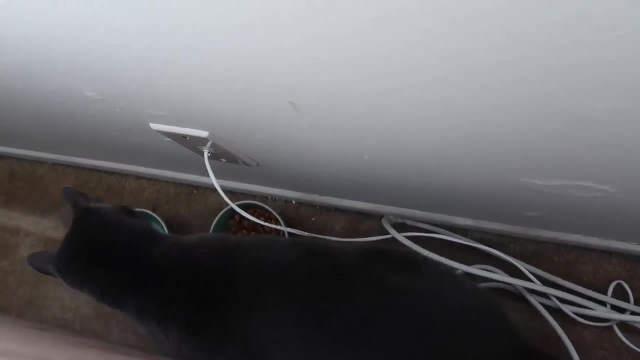 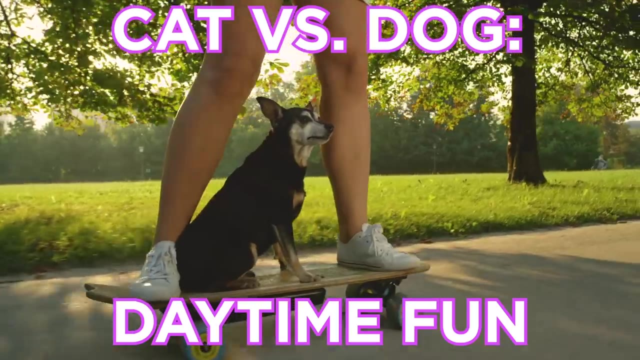 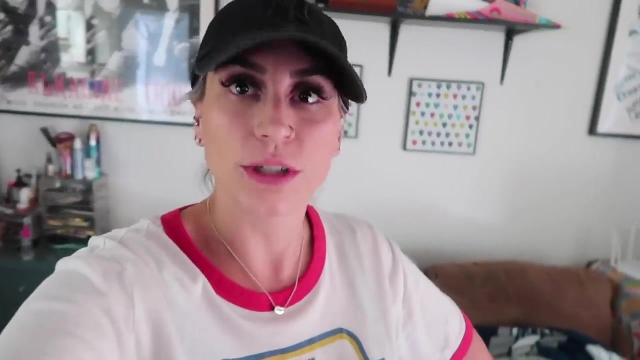 Y'all. I think this is a victory. She is eating and drinking. That's all I can really ask for at this point. This is a first for me. I'm gonna go run some errands, which means I'm gonna leave the house. 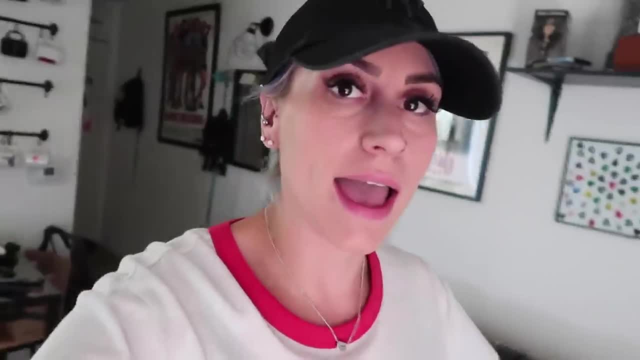 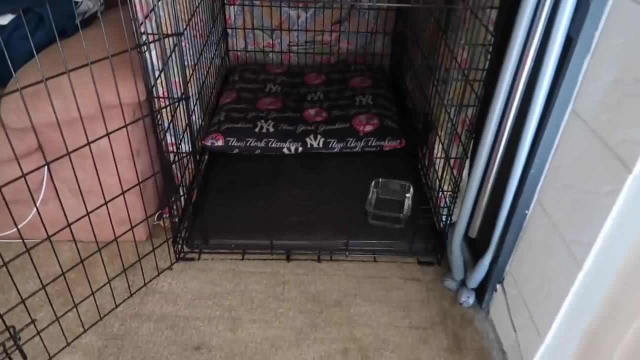 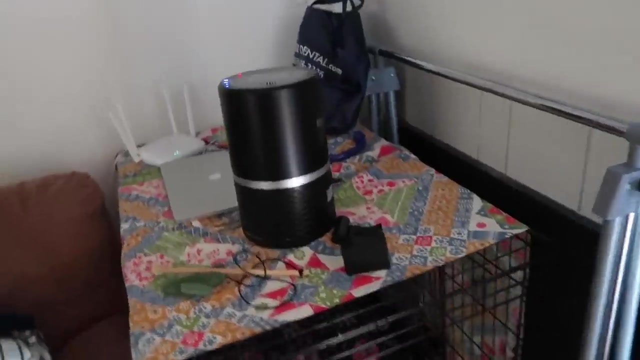 I feel like I'm forgetting something, cause normally I get Mabel all set up for her crate, So she has a big old crate, There's water and a pillow and sometimes her blanket. I have this little device which helps calm her down if she starts barking. 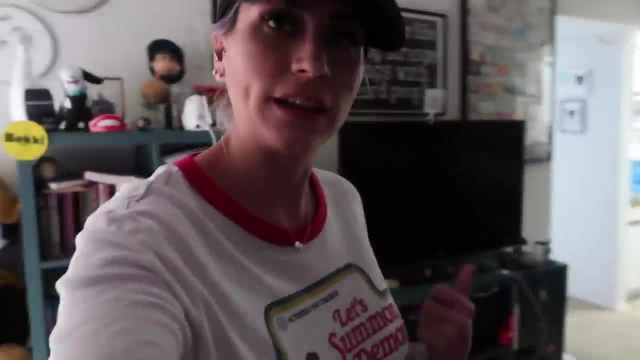 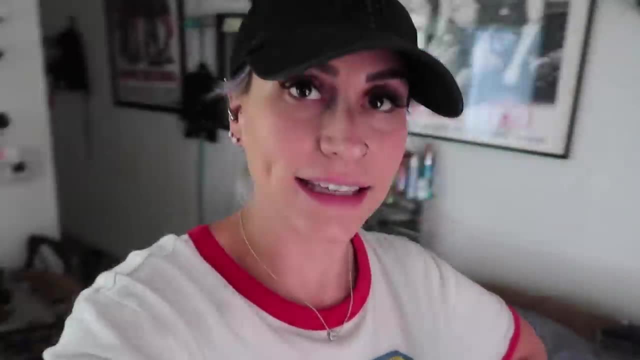 A camera system so that I can check in on her. I normally have to leave like a peanut butter or a Kong filled with peanut butter. I don't have to do that. The cat is just chilling, Still just there, going back and forth behind the couch. 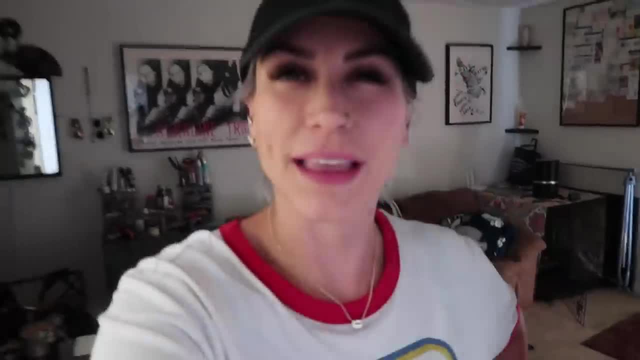 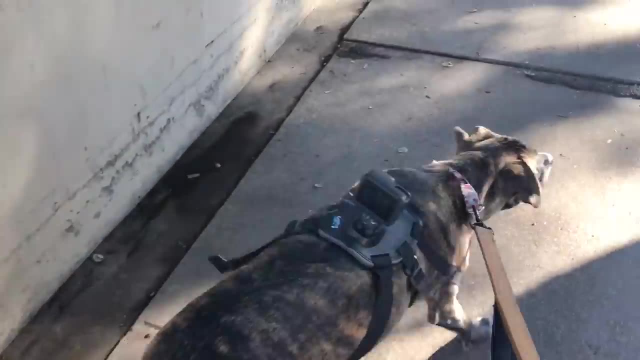 I don't know what cats want. I don't know what cats need. I think the point of them is that they don't really need anything. right, I didn't realize how much I missed having a dog. This is really nice. I will say, though, like it is a lot of work. 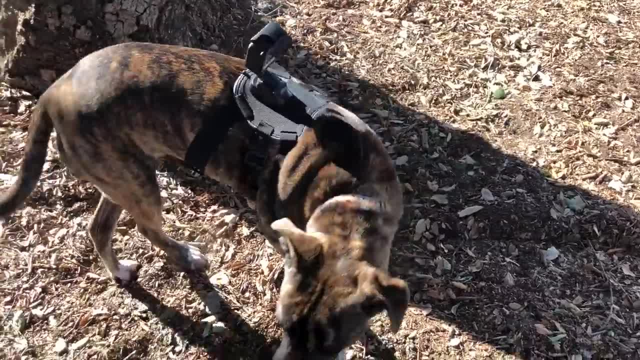 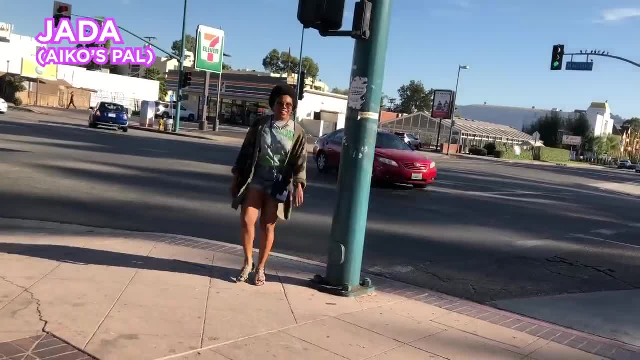 Much more work than mommy is. As much as I really like you, Mabel, I do miss my cat. I'm getting firmly pulled here. Okay, you're going a little fast. Hello, Hi, I have a dog, I know, I see. 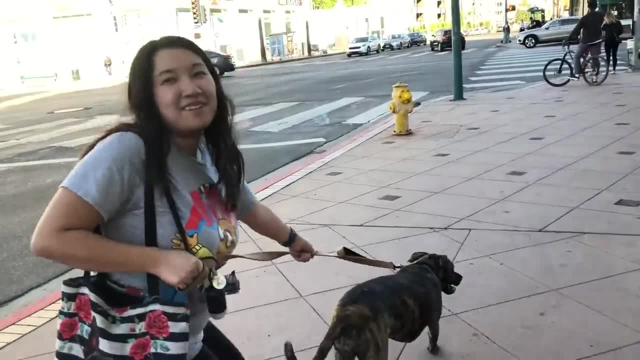 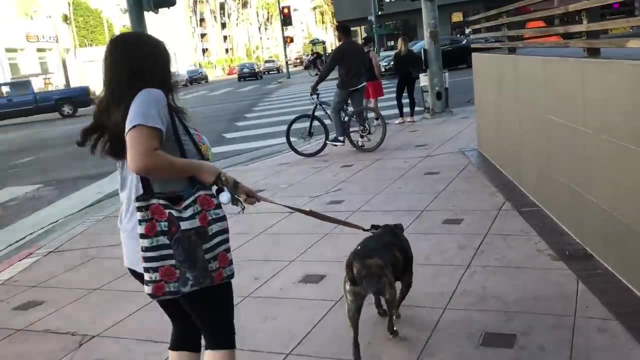 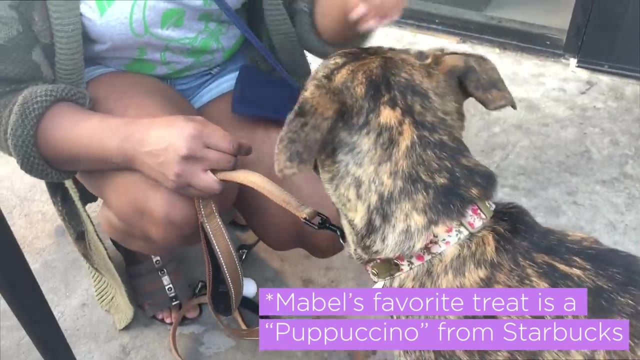 Her name is Mabel, Hi Mm-hmm. So I'm trying to keep her strong and keep her walking at the right pace. Do you need help, or I'm good? I'm good, You're good. Hi, Mabel, we're getting you a Puppuccino. 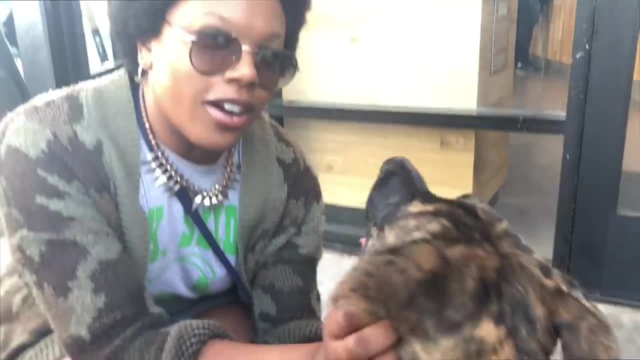 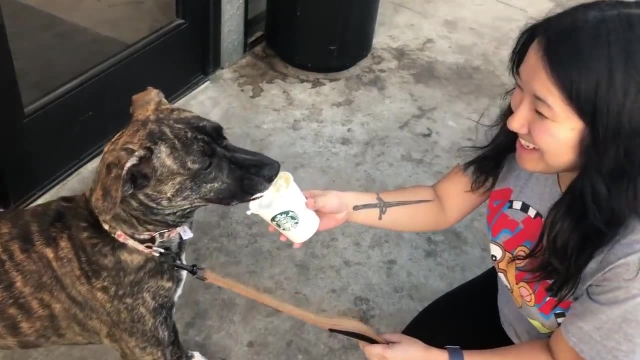 Can we talk about how much anxiety this girl has, Like you were gone for like three minutes and she was just screaming My gosh, she's getting it all on her mouth. I don't know what it would create. Is this okay? 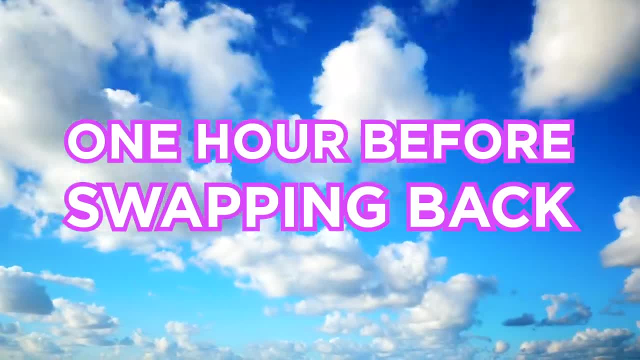 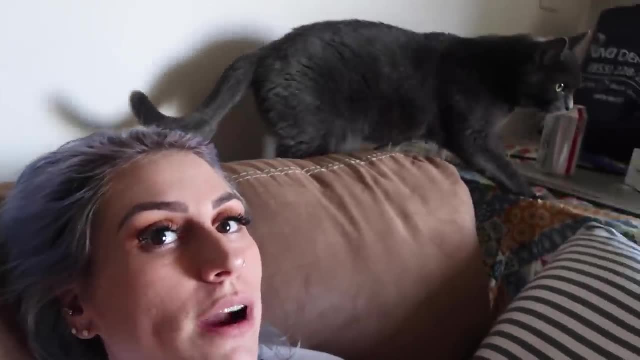 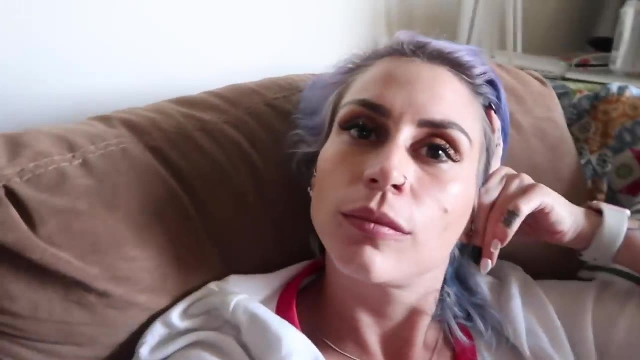 That was so full Two seconds ago. I'm not gonna lie, Mommy, this has been amongst the most boring 24 hours. Mommy's mommy is set to pick her up in about an hour, So mommy has decided to emerge. 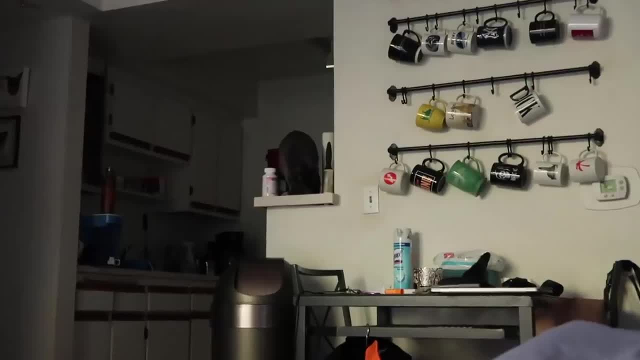 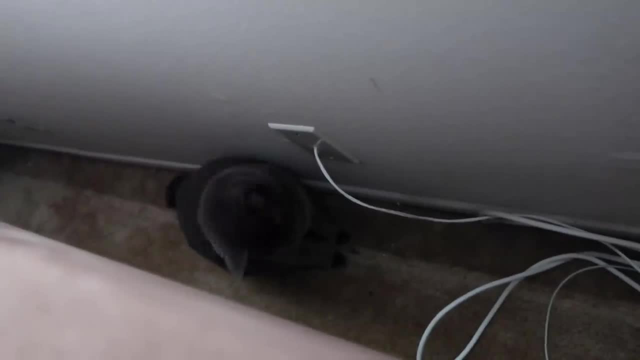 I don't get it. I don't get them. She got really brazen, really quick. Are you sad because I packed all your stuff? Yeah, Are you excited to go home? Yeah, I don't know what to tell you, baby. your mommy's on the way. 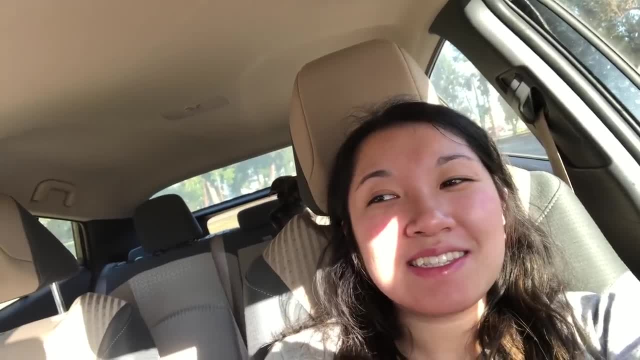 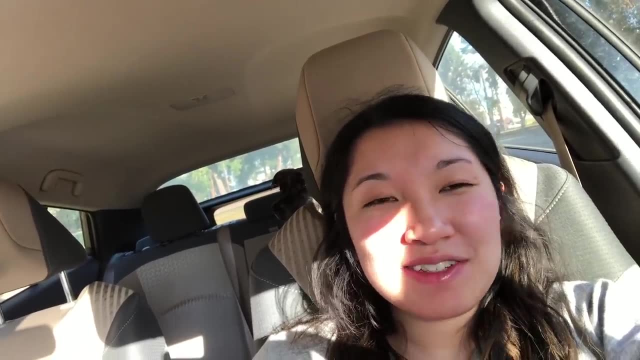 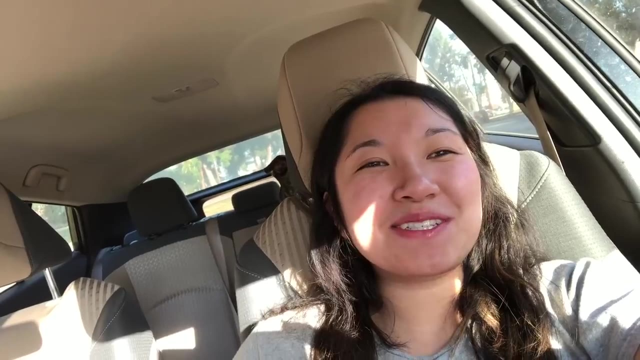 I think the thing that I've realized is that I, at least in the current moment, current stage of my life, I have to have a cat, because Mabel is beautiful and amazing. and a lot of work. I think this was successful. I think this was fun. You are welcome to.